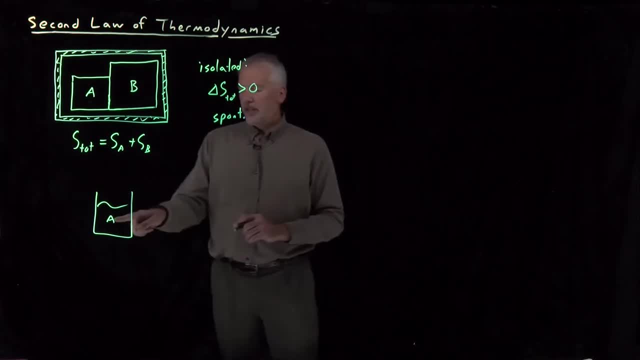 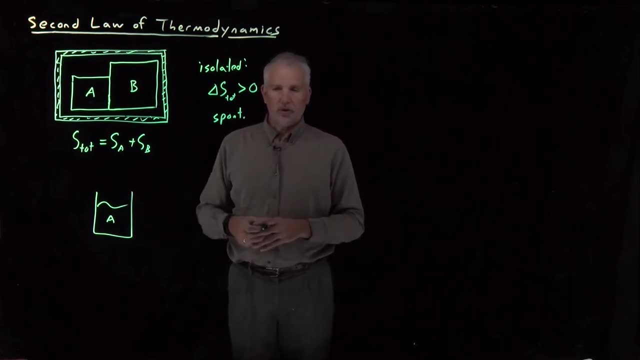 container. So in this case heat will transfer from the system to the surroundings, to the beaker that it's connected to, Or to the air above the solution, or to the broader room, or outside the room, the rest of the universe, all of the surroundings of the system. So normally we do things in conditions that are not isolated. 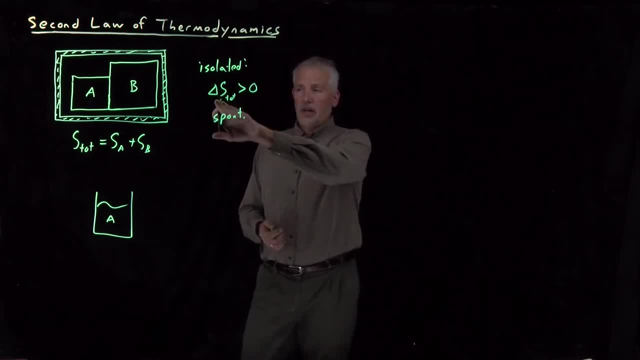 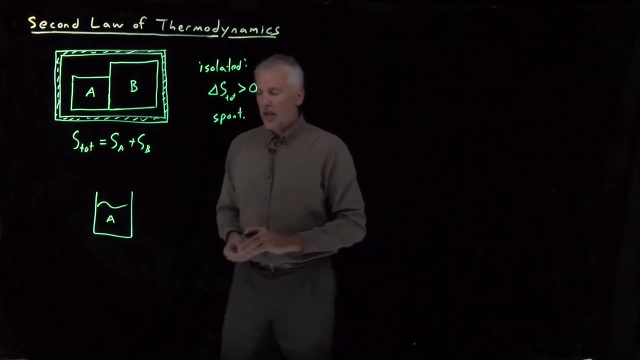 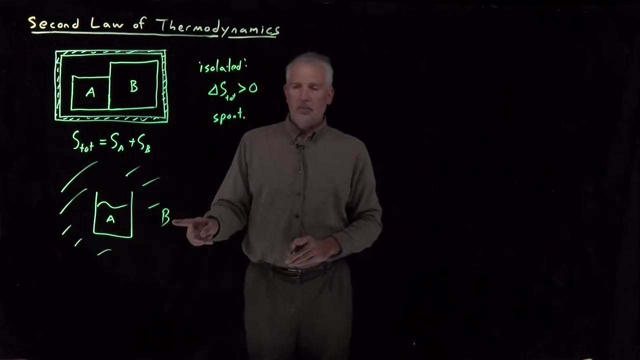 But it turns out we can still learn something useful about what the entropy says to us, about the spontaneity of a process, even for these non-isolated systems, because we can consider essentially all the rest of the surroundings to be this counterpart. So here's a picture of a system A. So in this case we had thermal transfer between part A and part B. 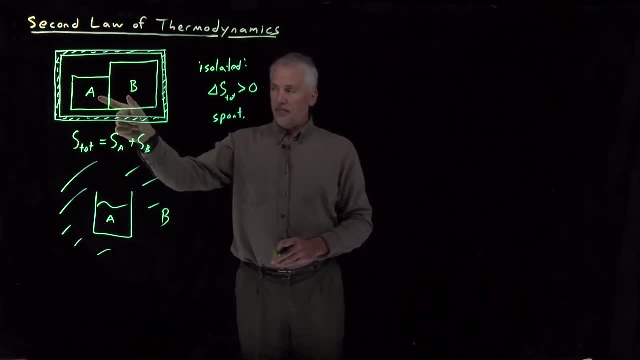 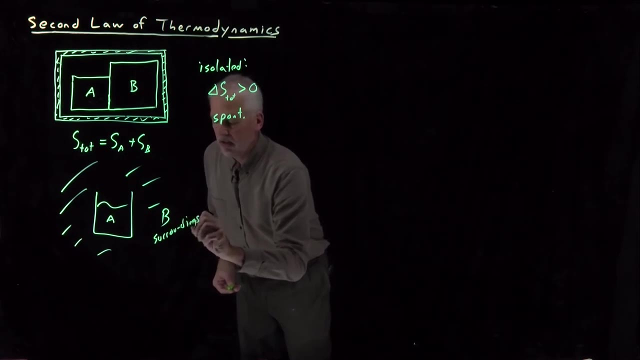 just no thermal transfer between those two parts of the system and the rest of the world. In this case, let's consider A to be the system we're interested in, B to be all of the surroundings, and together A and B make up the whole world, the whole universe, everything there is. 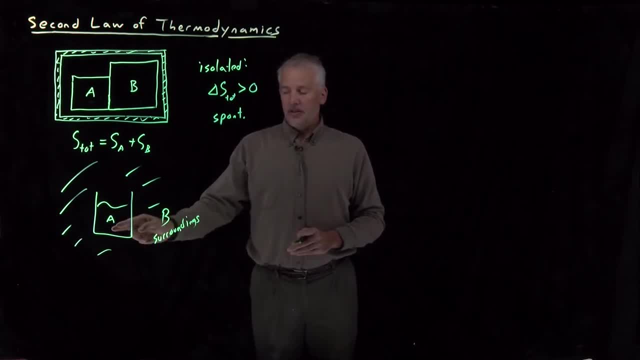 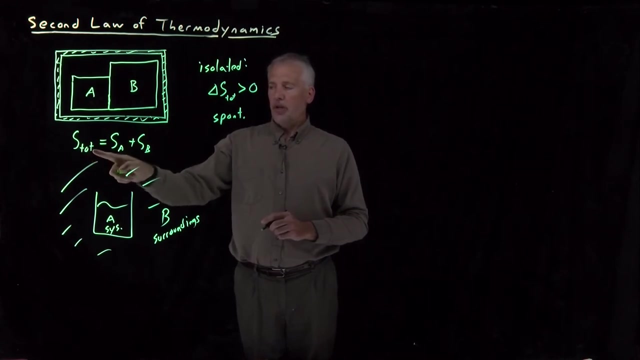 so in that case there's thermal transfer between the system and the surroundings, but there's no energy being transferred between the combined system, the entire universe and anything outside that. so the universe itself is thermally insulated from everything else. so in other words, where in this previous example we had the total energy- i'm sorry, the total entropy. 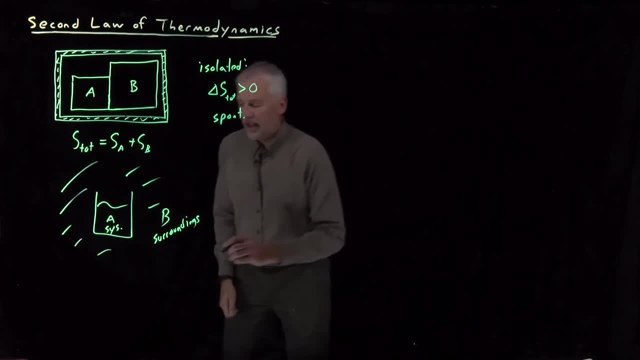 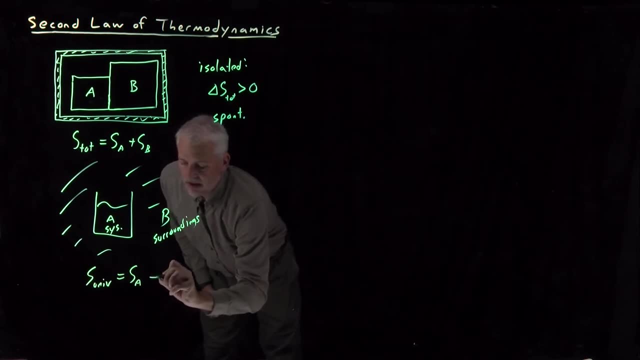 being the entropy of system a and the entropy of system b. here we can say the entropy of the entire universe is equal to the entropy of a, or the system, and the entropy of b or the surroundings. so system and surroundings together combine to make up the entire universe. 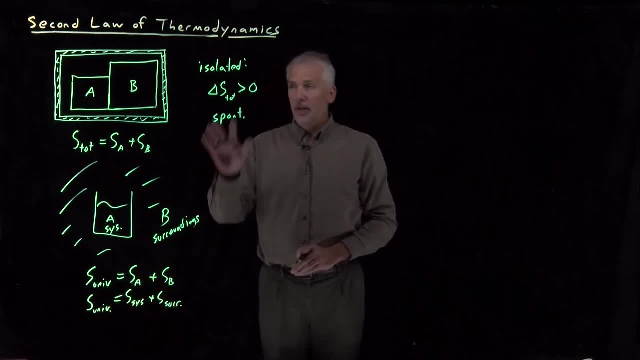 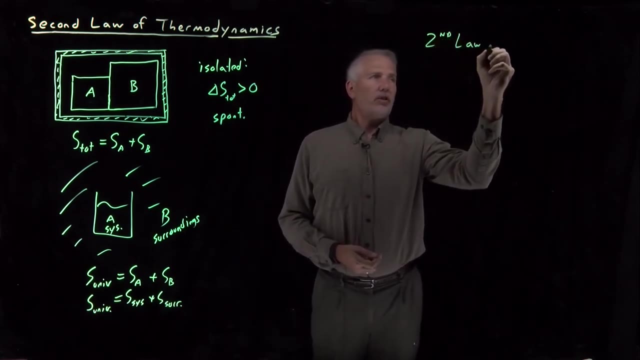 and the universe. the key observation is: the universe itself is an isolated system. it's thermally isolated. so everything that before we could say only about this isolated system, now we can say about the universe as a whole, and in fact that's an important enough statement that we call it the second law of thermodynamics. 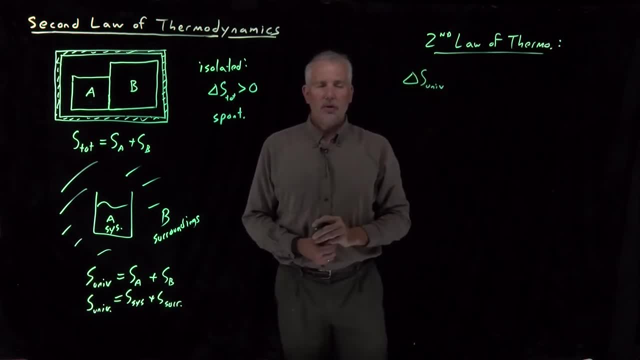 when the entropy change for the entire universe for a process is greater than zero. that's analogous to the entropy change for an isolated system being positive. that's going to be a spontaneous process. so if we can get enough information to determine that the entropy of the universe is increasing for a process, we know that process is going to be. 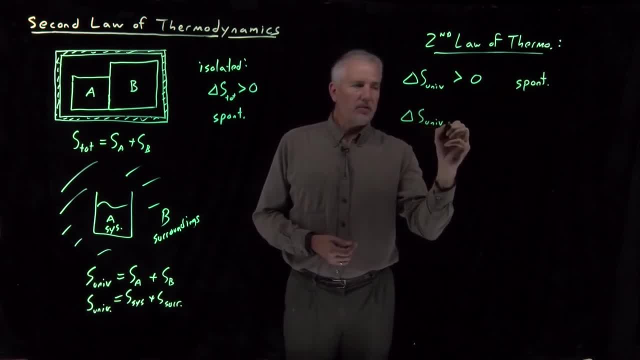 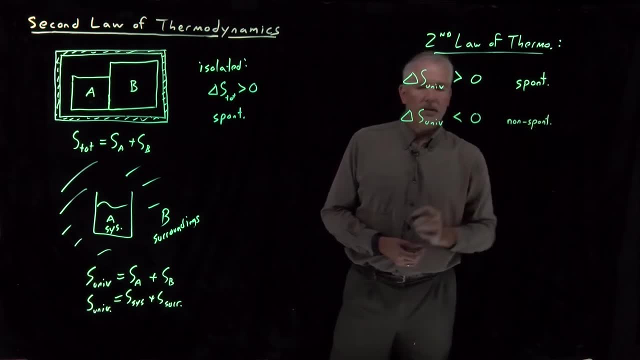 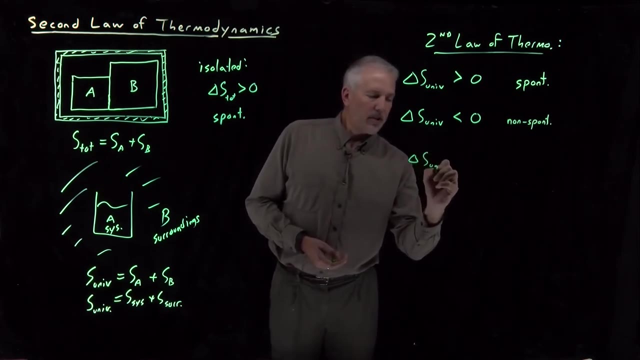 spontaneous. on the other hand, if the entropy change for the universe is negative, that'll be a non-spontaneous process. it won't happen. that's some process that is not going to happen. that leaves one possibility that we haven't discussed: what if the entropy change is equal to? 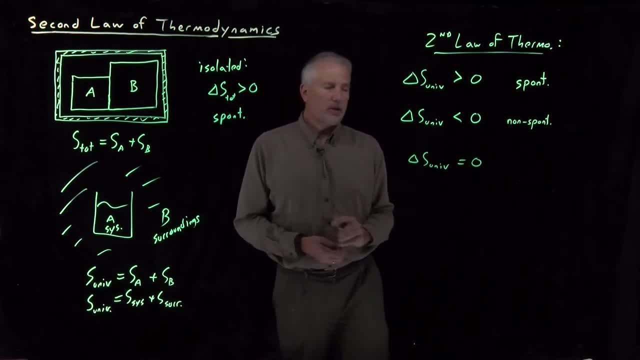 zero. if the entropy change is equal to zero for some process, we say that's an equilibrium process. essentially you could say that the process um doesn't care whether it does or doesn't happen if it. if it happens, the entropy change of the universe is negative. if it doesn't happen, or if it happens in reverse. the entropy change of the universe is is zero in all cases, so it doesn't matter whether the process happens or doesn't happen. in fact, what happens is the process is constantly happening: forwards a little bit, backwards a little bit, none of which is changing. 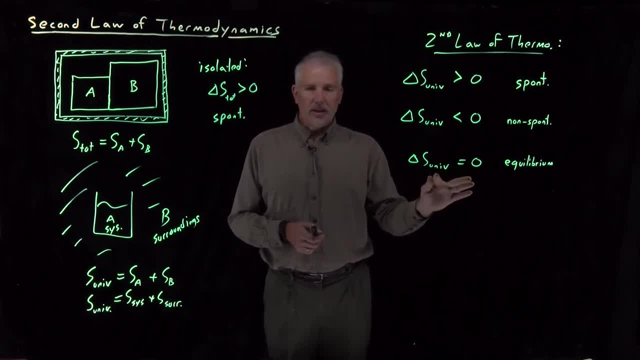 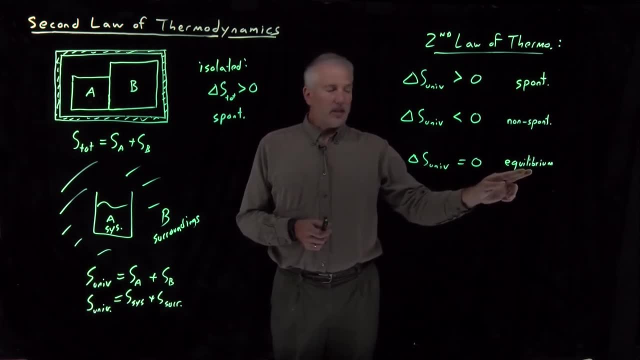 the entropy of the system, none of which is changing the entropy of the system, none of which is changing the entropy of the system, none of which is changing the probability of either one of those states. so, an equilibrium process. it doesn't matter whether state a or state b, the process happens, or 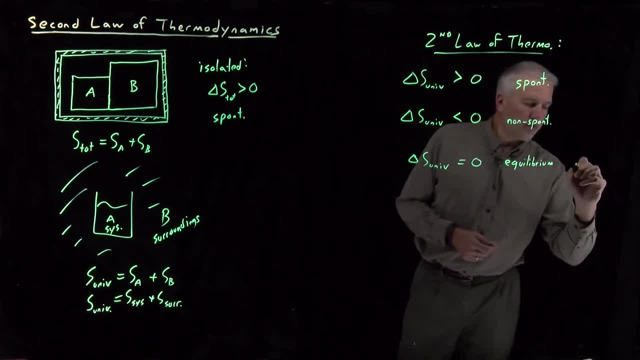 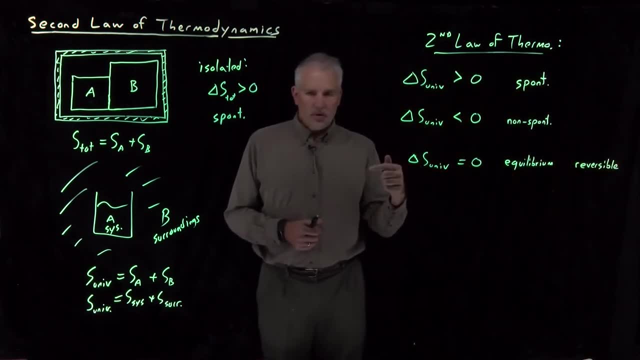 doesn't happen. so another word that we've used for an equilibrium process is a process that's reversible. that process happens forwards, backwards, can be reversed quite easily. the opposite of a reversible process is an irreversible process, of course. so a spontaneous process. process is going to happen spontaneously, like a marker falling due to gravity or a gas. 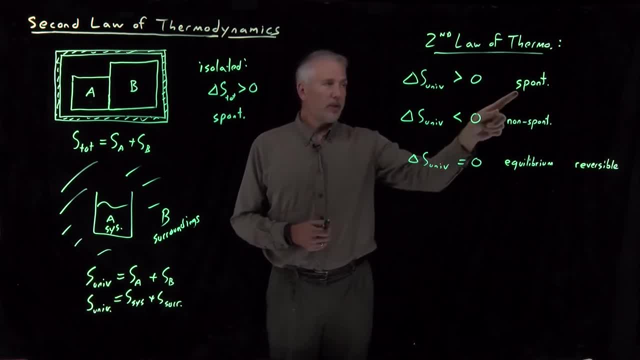 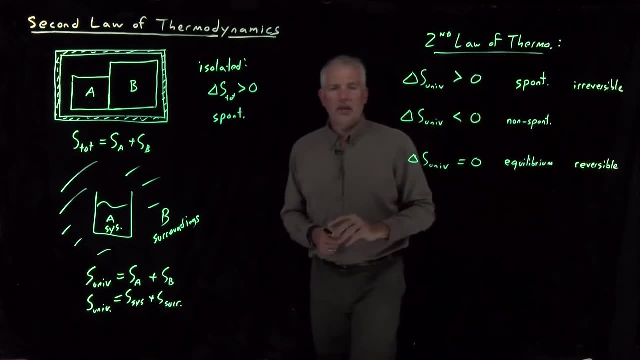 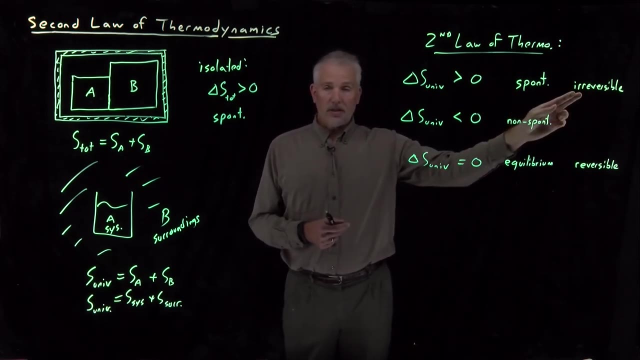 expanding to fill its container, or ice melting at room temperature. those spontaneous processes happen irreversibly. because it's spontaneous, the process is going to happen. once it's midstream happening, it's difficult to to turn that process around without a large input of energy. so that's an irreversible.